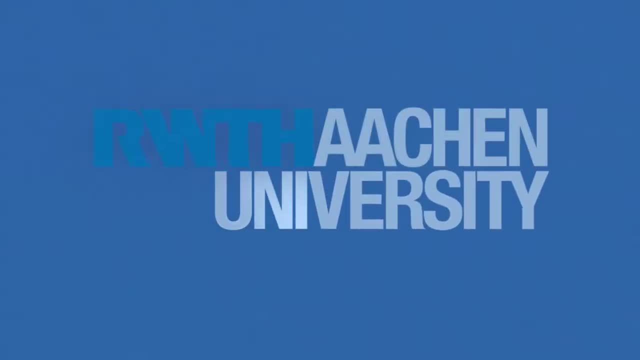 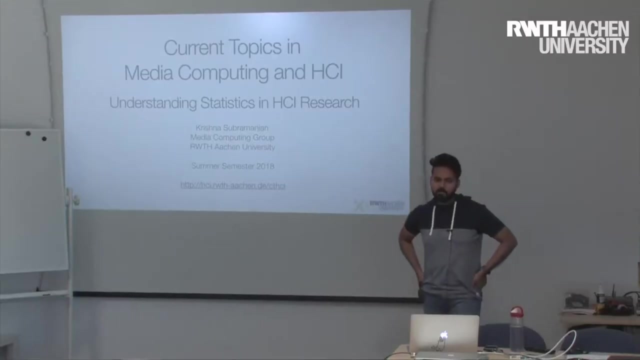 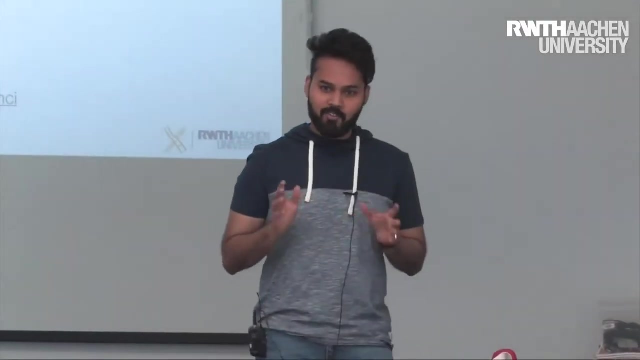 The following content has been provided by RWTH Aachen University. So today we'll be talking about statistics in HCA research. Might sound like a bit of a difficult topic, but trust me, it's actually really easy. I'm guessing you have all read some research papers. 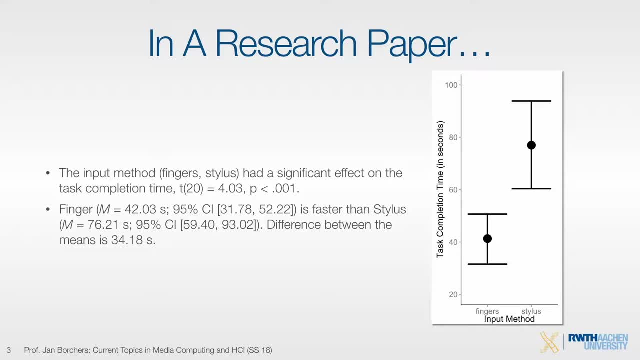 already, and in research papers you typically find under the results section content like this. So here we have. this is just made up, but you can find similar reports in your papers. So the input method- fingers, comma stylus- had a significant effect on the task completion time. and then they: 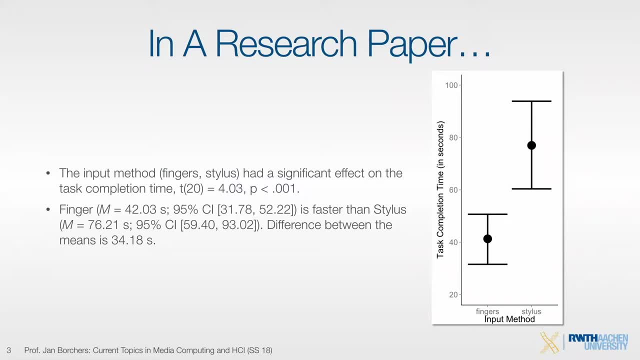 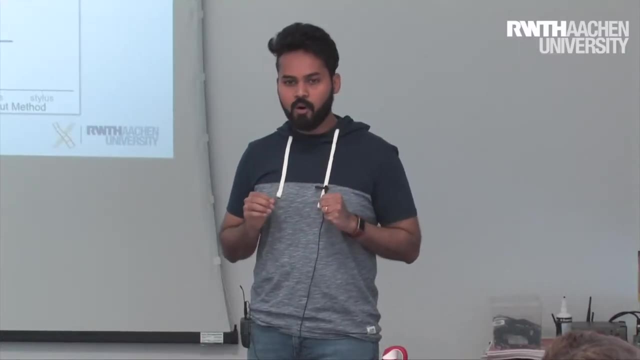 have a bunch of different notations and different numbers. So t of 20 equal to 4.03, p less than 0.001, and so on. So most of you probably don't know how to interpret this right And the objective of. 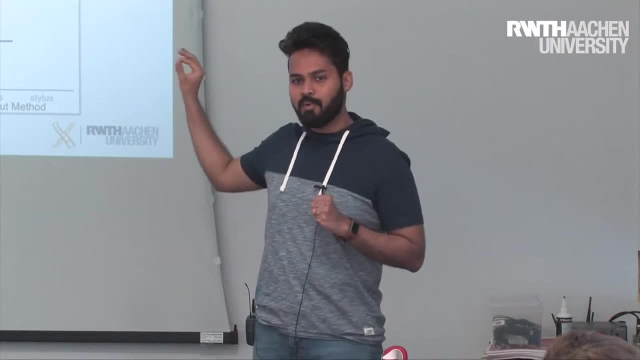 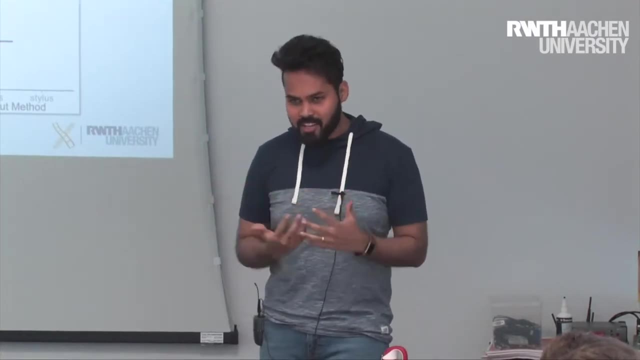 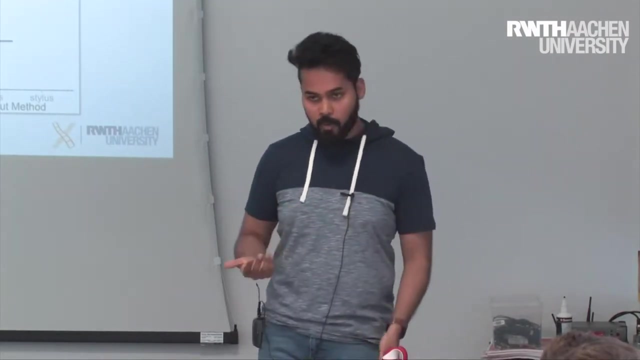 today's lecture is to help you guys learn and interpret such statements. So not just this statement, but similar statements that you can find in papers, Because teaching statistics from scratch is not feasible in one and half hours. okay, If you want to learn more about statistics. 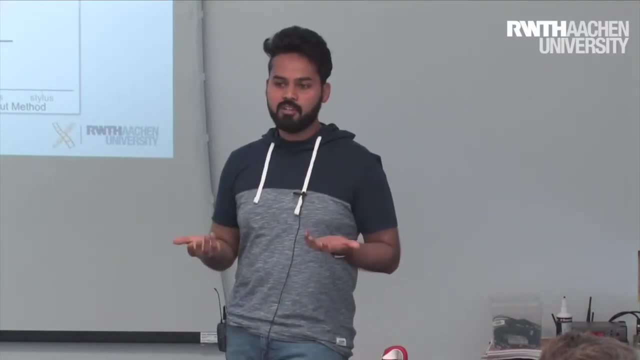 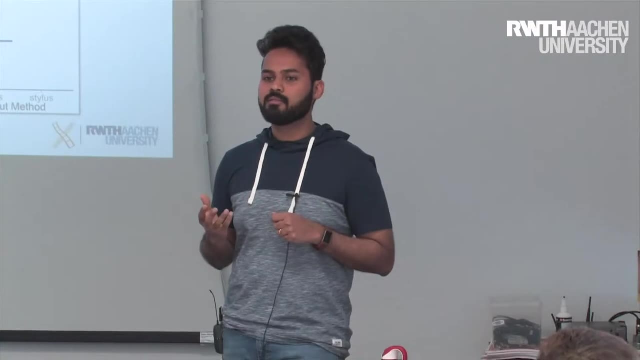 you can come up to me and I can suggest literature for it, But today I've just teach you how to interpret such stuff in papers and also the very fundamentals of how statistical analysis works. okay, There will be a lot of assume this, assume that in today's 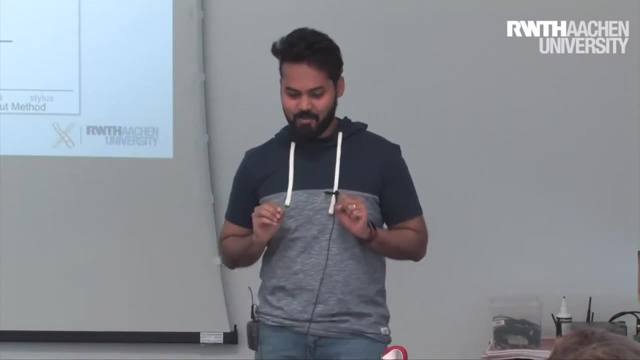 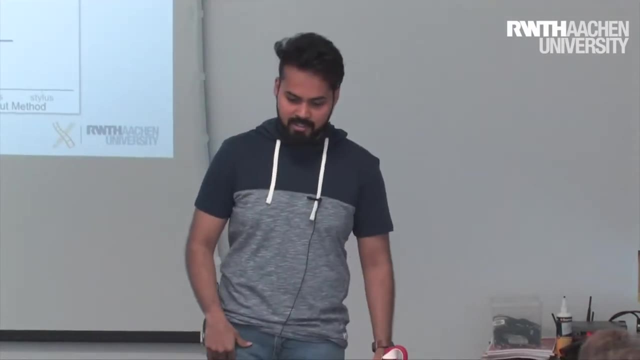 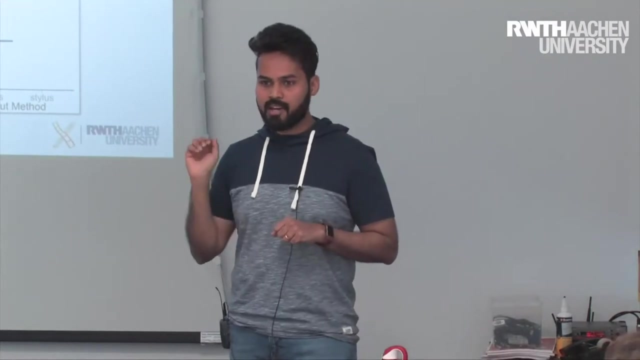 lecture. okay, So just trust me when I say you have to assume stuff, And we'll also look a bit at how to interpret graphs and you'll also have an in-class exercise based on this later on. So this is not just relevant for HCI research. okay. So statistical analysis: 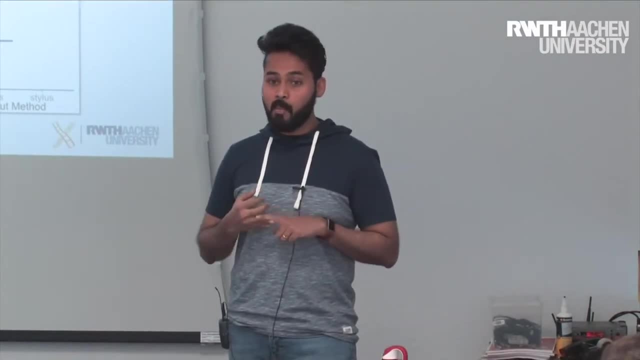 is quite commonly used in psychology medicine. So if you, if you take a look at Facebook feed, you can often find articles like: is coffee good for you? Is coffee gonna kill you? So all these are actually based on published research, but people don't know how to interpret the. 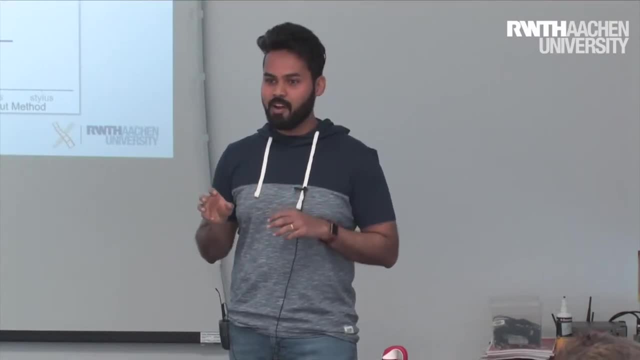 research section, so they just make it into a fancy headline. okay, But hopefully today, after learning what you will, you will be able to read those research papers for you and you'll be able to interpret them. So thank you very much for your attention. 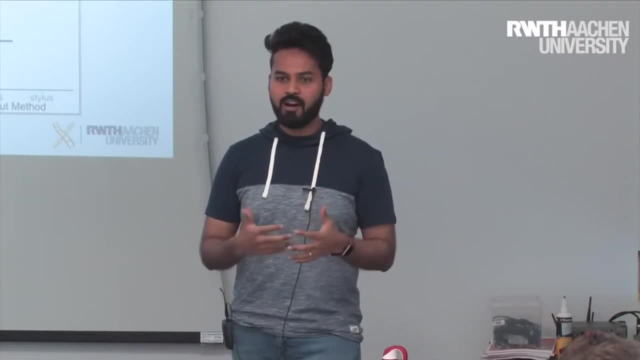 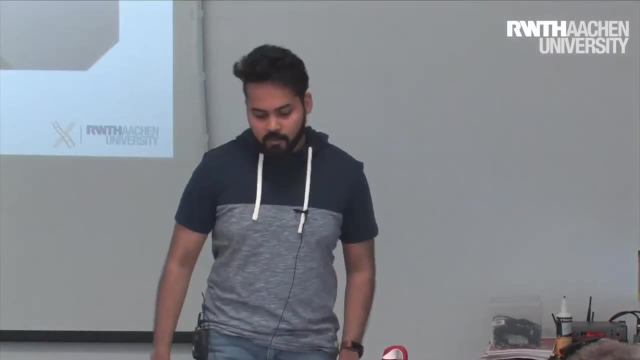 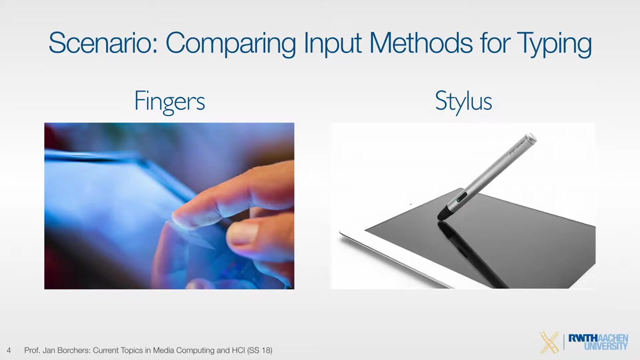 yourself and you can understand it. okay. You don't have to rely upon headlines anymore. you can make your own interpretations, okay. So for the purpose of today's lecture, let's consider a very, very simple scenario. So you are comparing input methods for typing on. 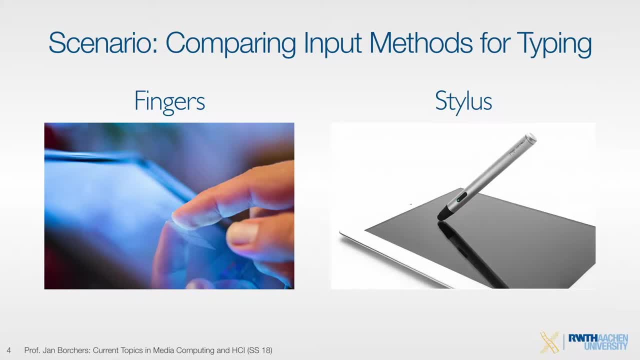 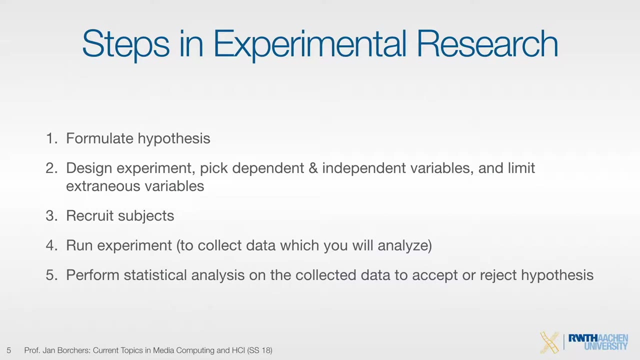 touch screens So you can either use your fingers or you can use a stylus. okay, So assume there is a keyboard, a virtual keyboard, and then you can either use your fingers or stylus for typing. So here are the steps in experimental research. So if you want to conduct an experiment and if you want 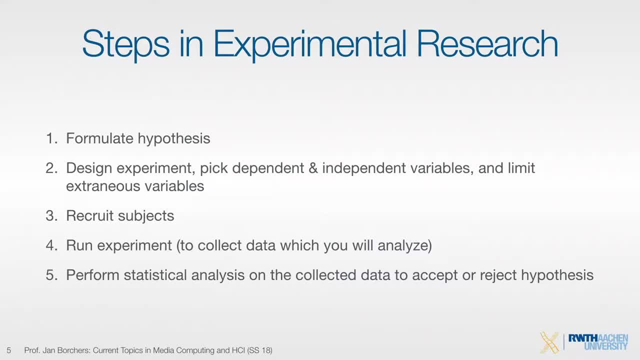 to show that using stylus is much faster or more accurate than using fingers, or the other way around, then you have to conduct an experiment right. So these are the steps in your experiment. So the first step would be to formulate hypothesis. The second step would be to design the experiment. 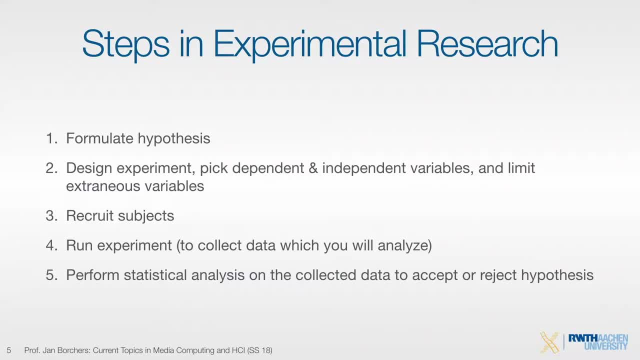 pick the dependent and independent variables and limit the extraneous variables. The third step would be to recruit subjects or participants. The fourth step is to run the experiment, And the last step, and the crucial step that we'll be looking at in more detail today, is performing statistical 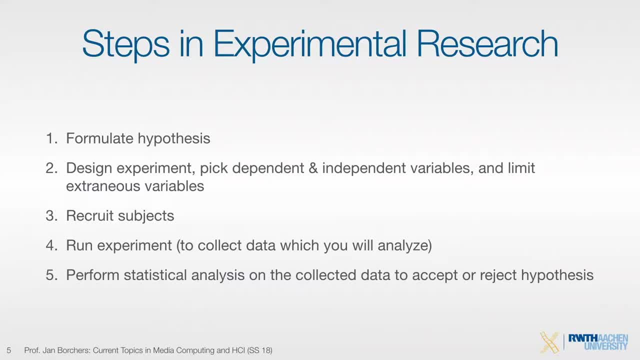 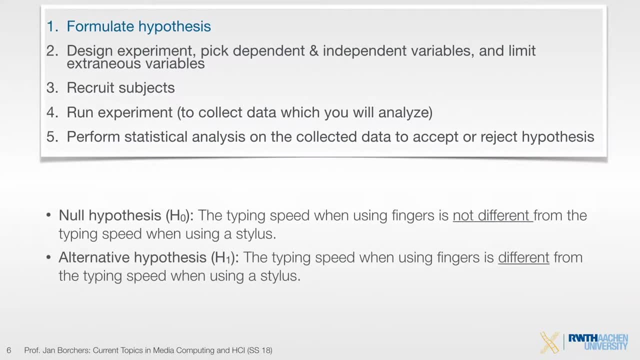 analysis on the data that you have collected. So let's go through it one by one. So first step is formulating hypothesis, and you have what's called a null hypothesis and an alternative hypothesis. So these are terms that you should already be familiar with, right? So null hypothesis. 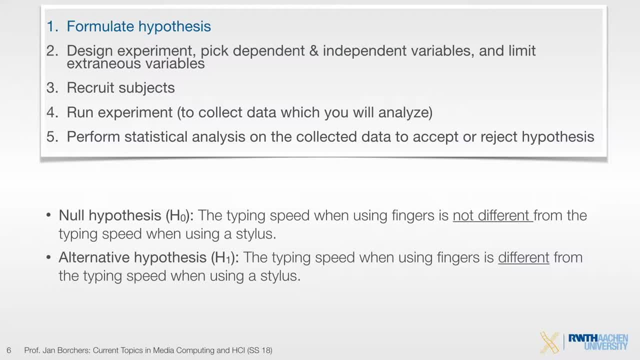 between the two conditions. So this is what we know currently, this is what we are trying to disprove, right? And then the alternative hypothesis would be the opposite of that. So in this case, the null hypothesis is that the typing speed when using fingers is not different from typing speed. 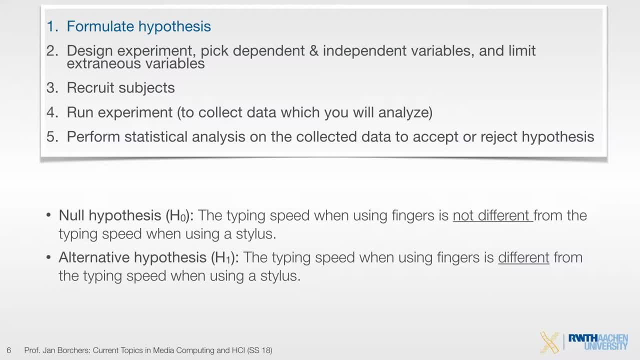 using a stylus. okay, So this is what we currently know about the world before conducting our experiment, and this is what we are trying to disprove, And the alternative hypothesis is what our hypothesis is basically. So the typing speed when using fingers is different from the typing 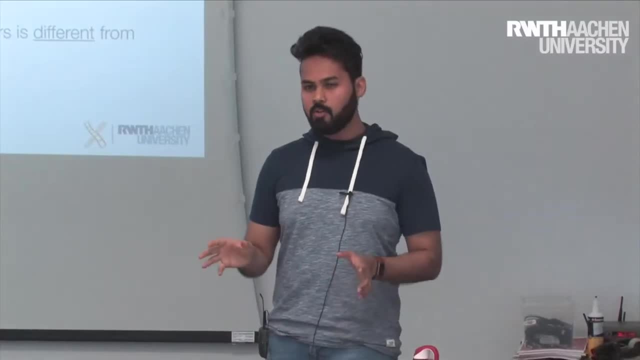 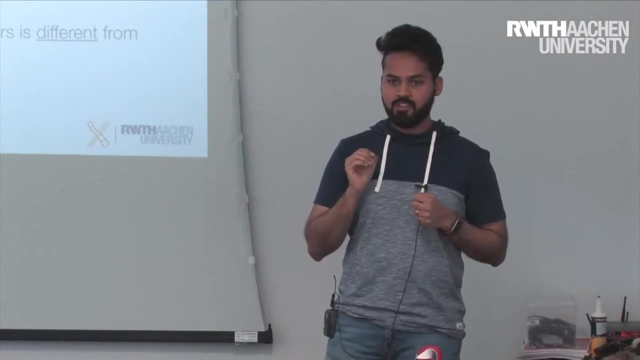 speed when using a stylus, okay. So one thing you will notice about statistical analysis is it is not a very aggressive approach, it is a very defensive approach. So you always try to assume that everything is going to go wrong with what you're doing. And then, even with that assumption, 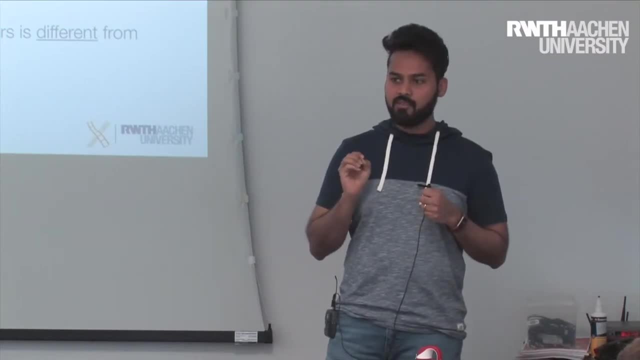 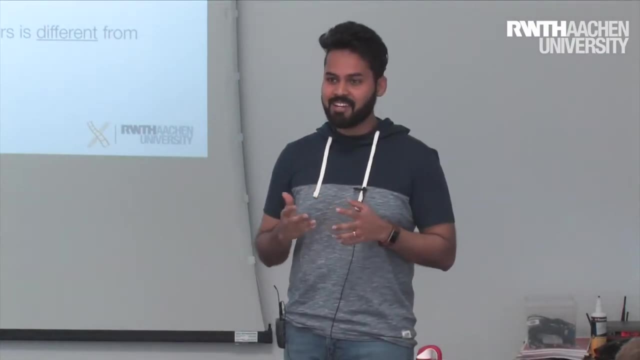 can you still get a significant finding? Okay, so it is a very defensive, very circumspect approach, as it should be, because you don't want to find things that are incorrect because it could affect a lot of people, right, I mean yes. 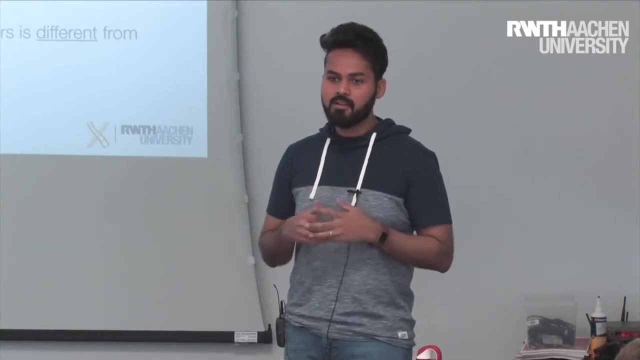 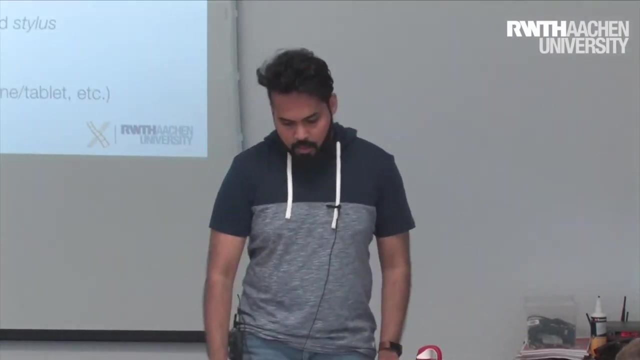 if you find that using stylus is faster than using fingers and if it is incorrect, maybe it's not a big deal, But in medicine and in psychology this could lead to you know difference between life and death. So it is very circumspect And the second step is designing an experiment. So in 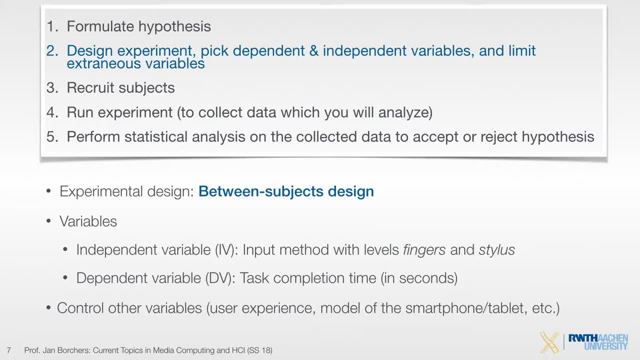 this case you could choose a between subjects design and you have certain variables. so the independent variable here would be the input method that the user uses, so either fingers or stylus, And the dependent variable is the task completion time, because that's what you want to show in your hypothesis. It could also be error rate or something. 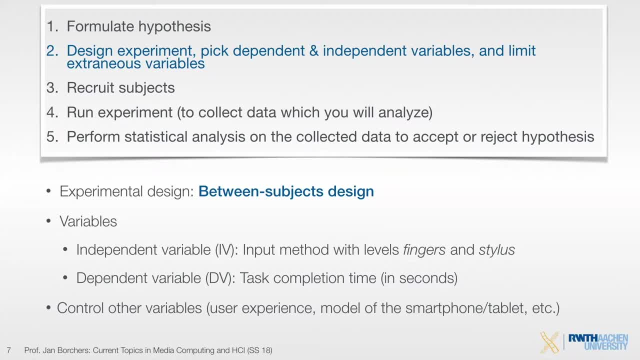 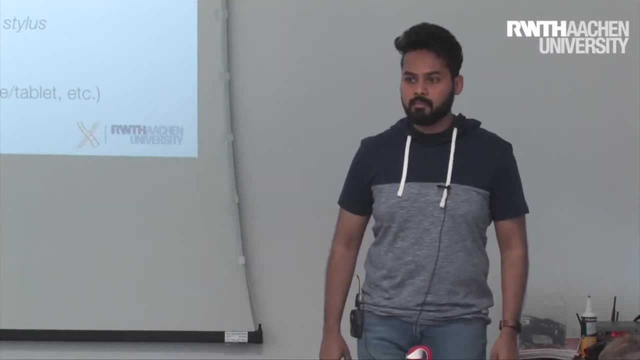 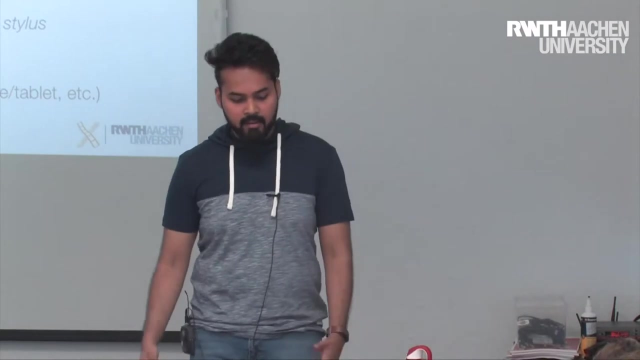 depending on your hypothesis, And, of course, you will want to control for other variables. Why are we doing this? Why do you have to control for user experience, for example? Because it might potentially influence our results Exactly. So you want to show that the input method causes the change in task completion time. 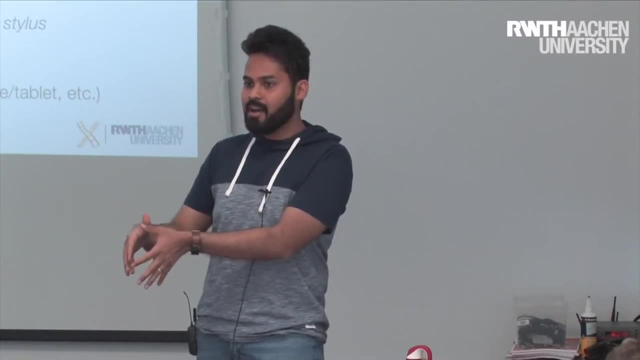 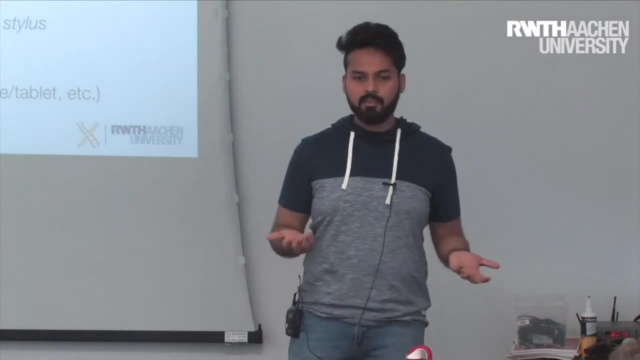 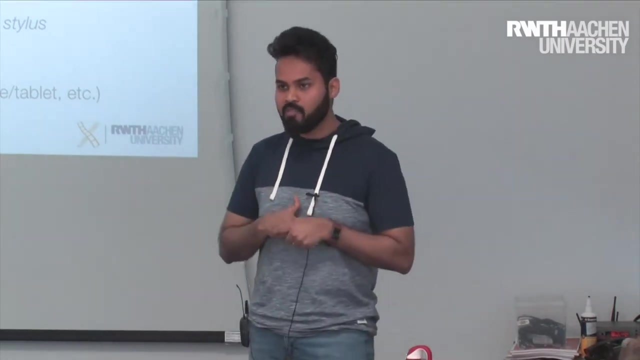 So either it increases the task completion or decreases the task completion time. So you want to limit or keep other variables as constants, Okay, so this is something that researchers spend a lot of time about, So they need to think about what are the possible confounding variables. 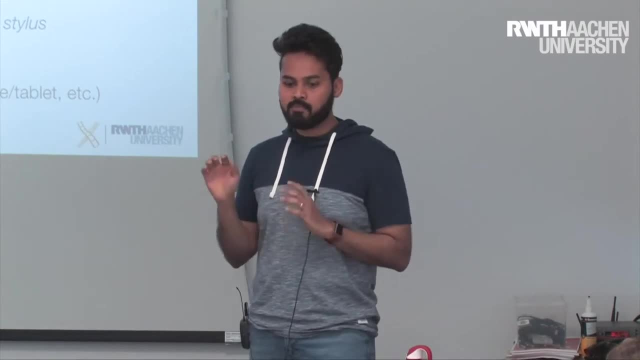 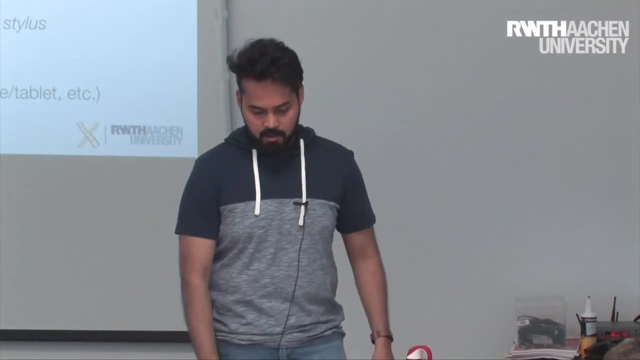 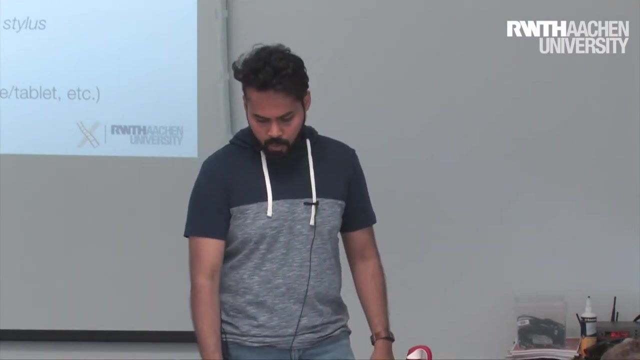 or extraneous variables and they need to try and keep them all constant or limit them in some way. So in this case, yeah, it'll be user experience model of the smartphone, tablet and so on. Maybe the text that the user is typing that needs to be kept constant as well. All right, and you? 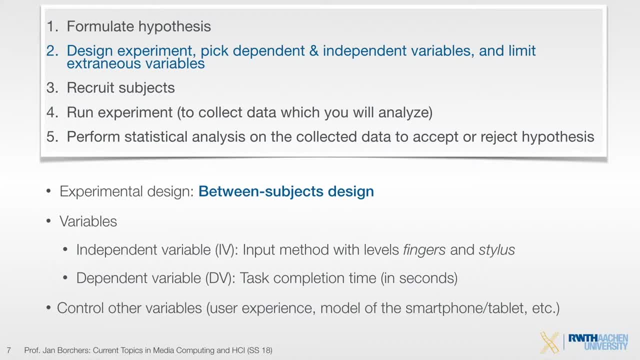 recruit subjects. If the task is going to take a lot of time, it's going to take a lot of time. then you bribe them with with sweets or something like that, And, yeah, they participate in your study. and then you run the experiment and you collect the data, And then we come to the last. 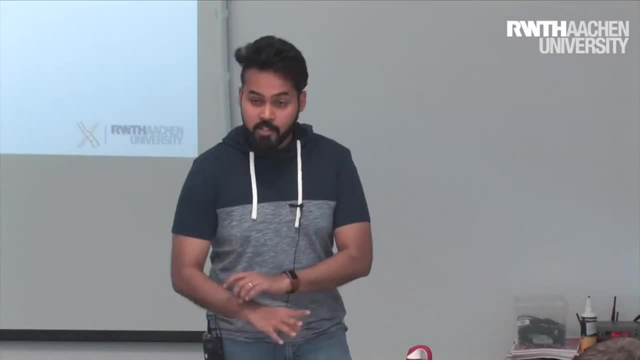 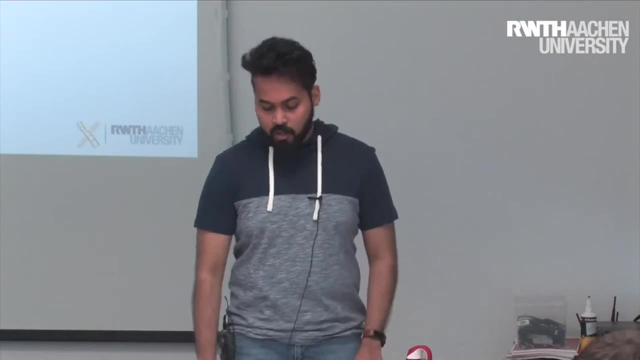 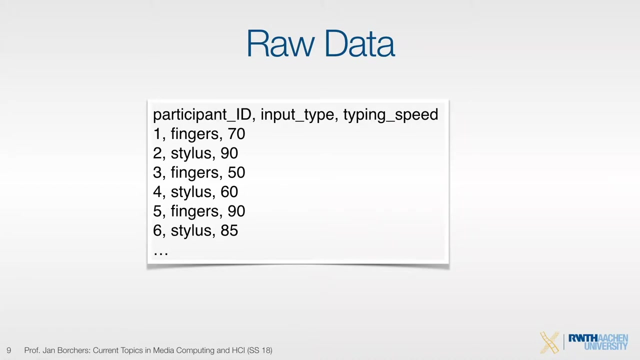 step, So performing statistical analysis. So let's assume you have done the experiment. now Let's assume you've had like 30 users for your study and you've collected data. So the data is going to look something like this, right? So this is a CSV file, comma separated value file, And you 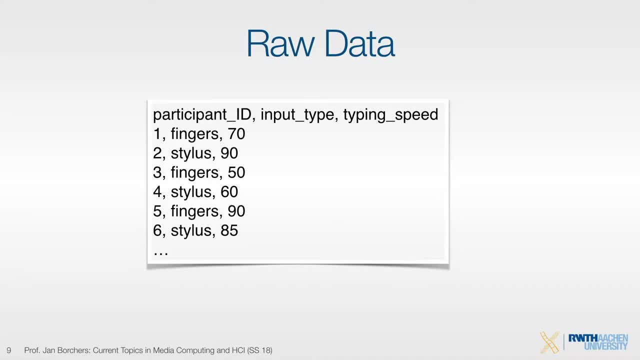 will have the participant ID, you have the input type, which is the independent variable, and you have the typing speed, which is the dependent variable. So why don't we just analyze this? Can you, by just looking at it, tell me something that you notice? Can you, for example? I mean, 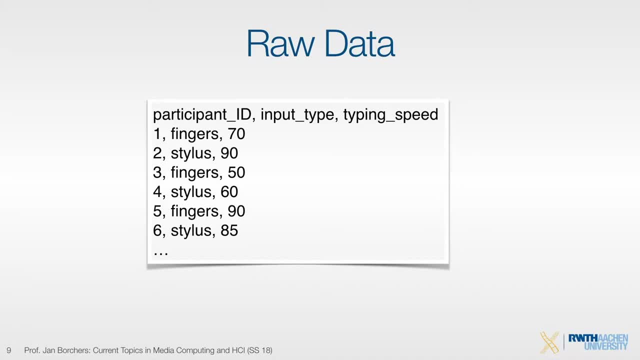 assuming that the CSV file is completely shown to you. I have cut off most of it. would you be able to see if you can see that the CSV file is completely shown to you? Would you be able to see that the CSV file is completely shown to you? I have cut off most of it. Would you be able to see? 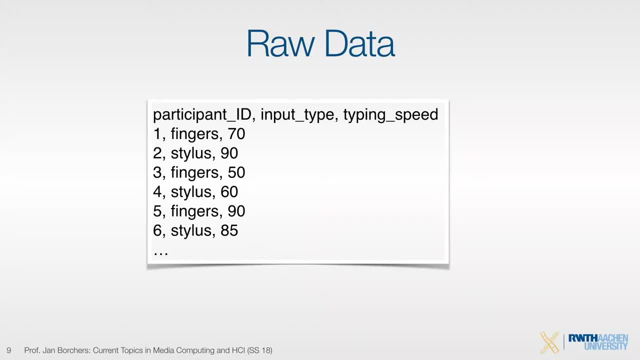 whether the fingers condition resulted in more typing speed or not. No, Yeah, So this is tabulation. This is textual data, right? So we humans are not good at noticing patterns in text. It is very hard to get a summary of the data. It is very hard to see the spread of data. 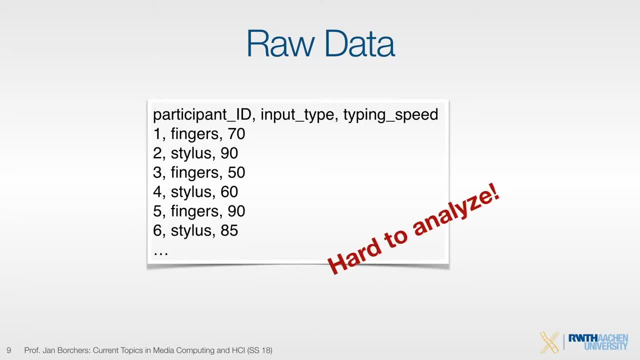 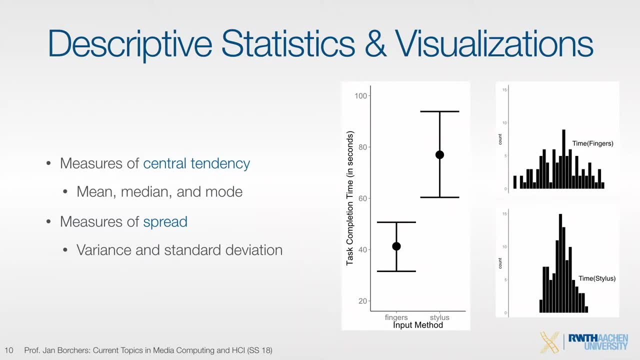 So it is very hard to analyze by just looking at the raw CSV file. So we use descriptive statistics and visualization. So descriptive statistics are ways to summarize the data. So one standard measure of descriptive statistics is the mean. So if you say that the 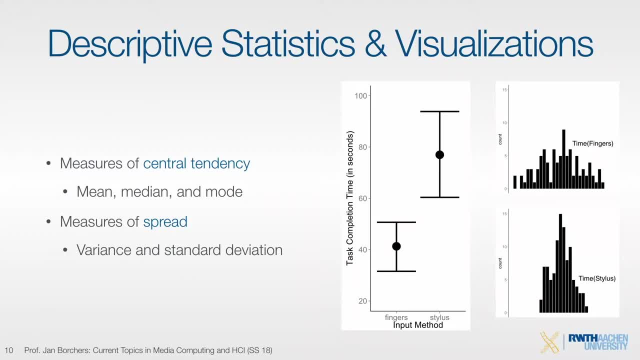 mean of the stylus condition is 30 words per minute and the mean of the fingers condition is 60 words per minute. this is easy to compare, right? Or easier to compare Because you're not looking at the entire bunch of data, you're just looking at one data, So you can see that the 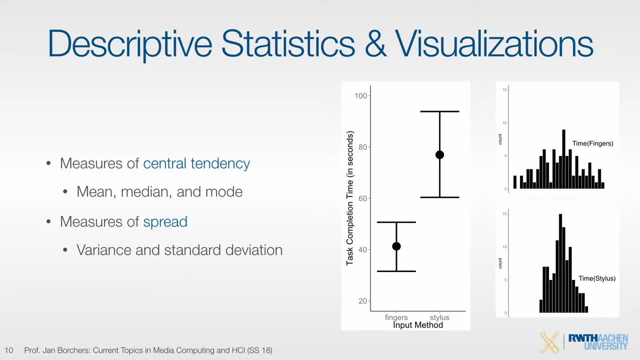 mean of the stylus condition is 30 words per minute and the mean of the fingers condition is 60 words per minute. So you can see that the mean of the fingers condition is 60 words per minute. So you also have median. you also have mode, So each of these are used for different types of 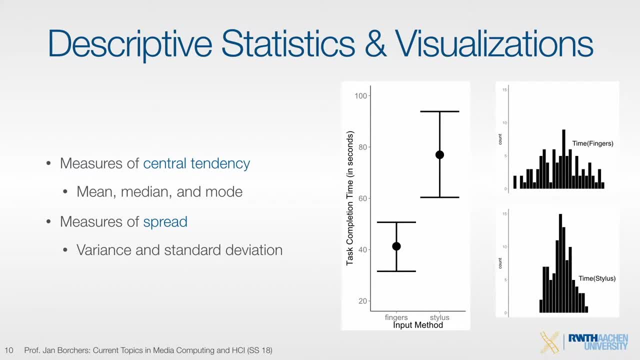 data okay, But they're all measures of central tendency, So a single value to represent the entire distribution. And you also have measures of spread like variance and standard deviation, which tell you how widespread the data is. So, if you say the standard deviation of my distribution. 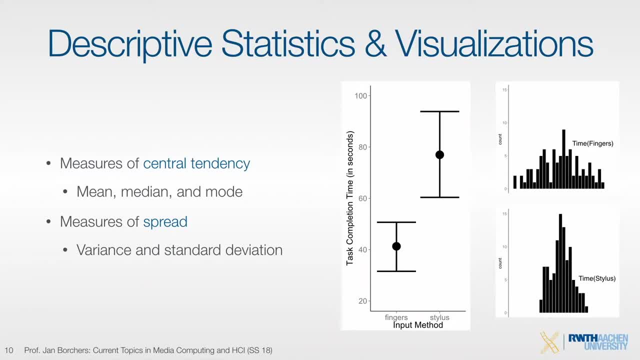 is 5 versus the standard deviation of 10, then standard deviation of 10 means the users had more varied typing speed. okay, So that's what it means, And you also use visualizations to represent this better. So here we have a very simple box. 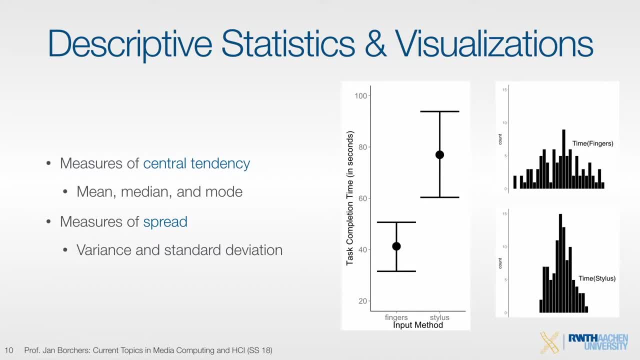 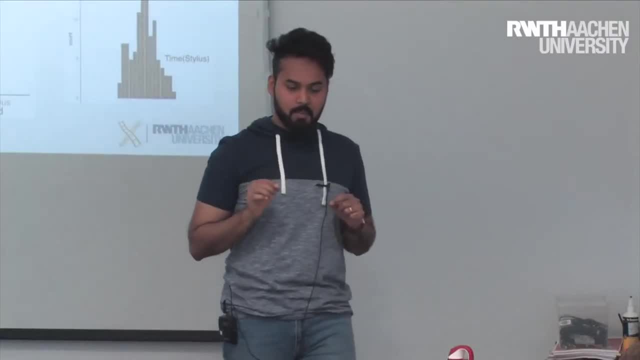 plot. well, a minified version of a box plot, You have the mean of the two distributions and this is what's called an error bar, which you will learn a bit about later today, But it basically shows how widespread the data is. 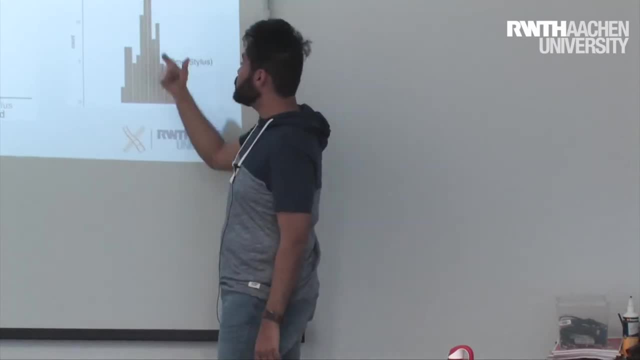 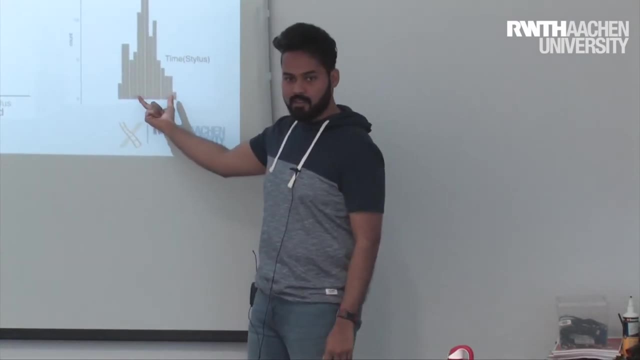 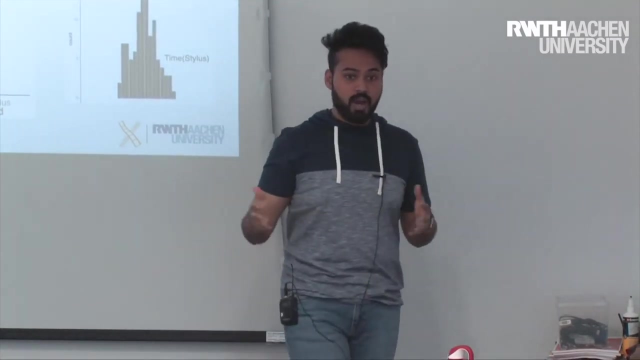 Okay, And here you have the spread of the data. So from here you can see that the stylus condition, it has less standard deviation, it has less variance, So users are more consistent in using the stylus condition, whereas with fingers users were much more widespread. So you had users. I don't. 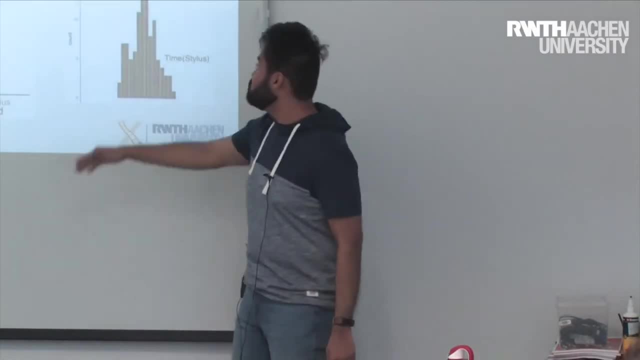 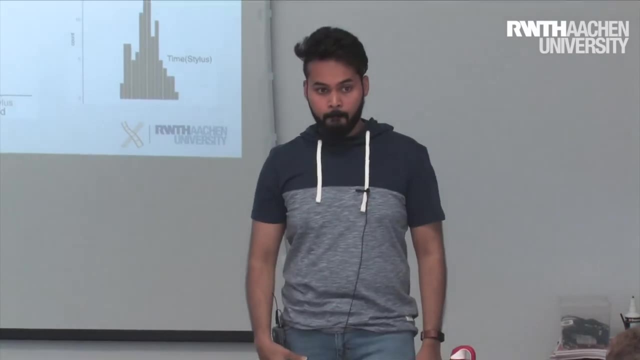 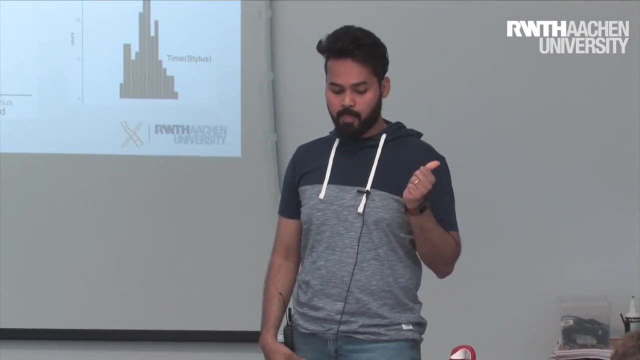 know typing at 10 words per minute, all the way to users who typed at, I don't know, 250 words per minute. So data is more widespread over there. Mode is the value that repeats most often, So for certain types of data you will report mode as the. 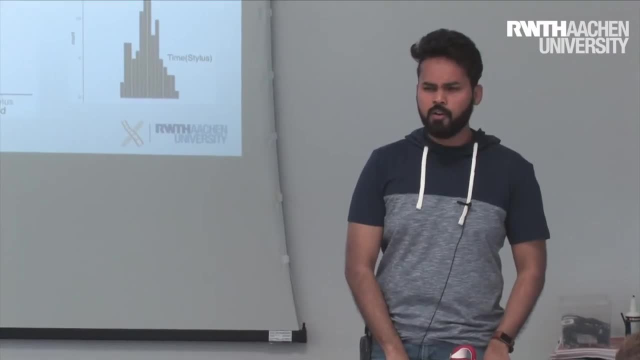 measure of central tendency. So do you guys know what a Likert type scale is? You all probably know, but you just don't know that it's called this way. So often in questionnaires you have questions like: please rate this from 1 to 5.. 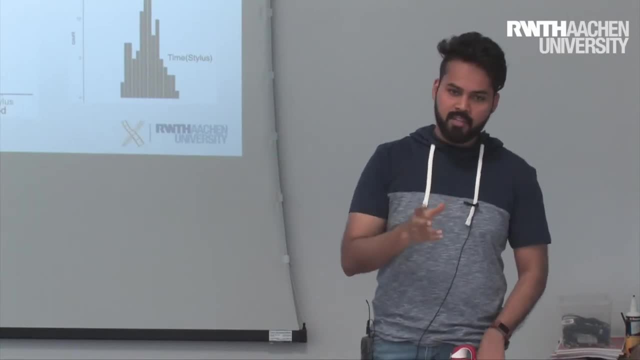 1 being the most and 5 being the least or whatever. So they have these rating scales right. So these are called Likert type data, And over here it doesn't make sense to compute the mean. It makes more sense to compute the mode or the median, for example. So for certain types of data you will 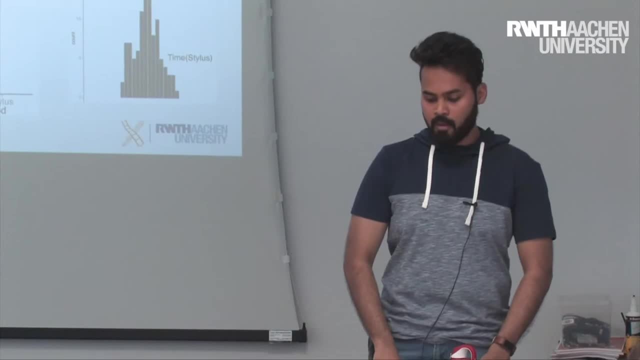 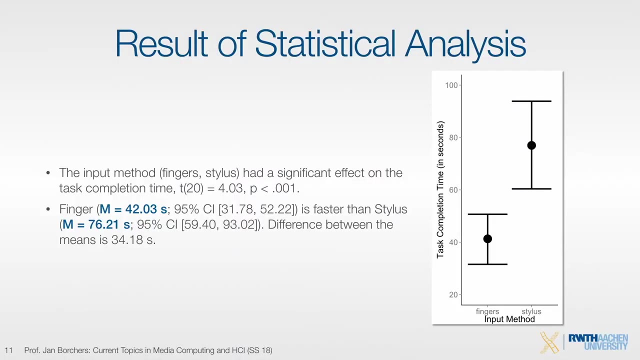 change your central tendency, your measure of central tendency? Yeah, But in most cases you will end up using mean. With that, you'll be able to interpret this part of the results. So we're just getting started, So you'll be able to find that a. 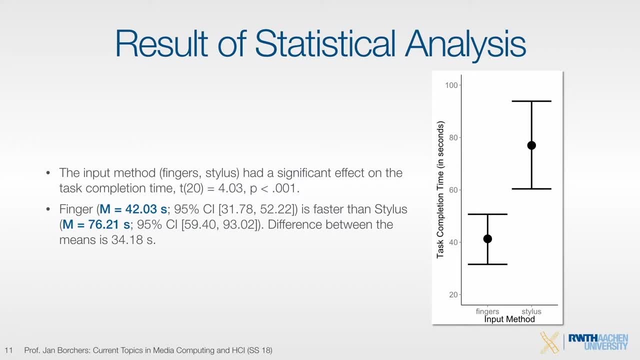 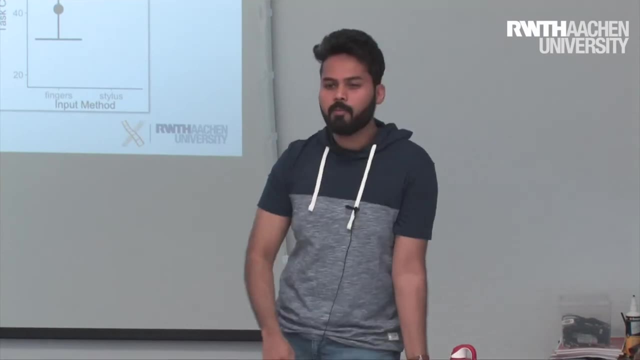 lot of research papers. in the results section, they report the mean of the distributions. Some would also report the standard deviation, Some don't, But most of them should report the mean, So you'll be able to get that now onwards. So what's the problem, though, with descriptive statistics? 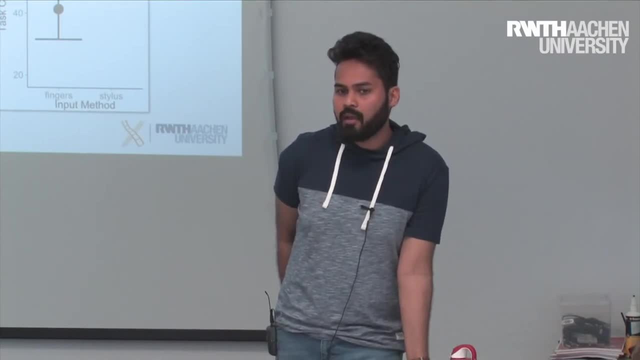 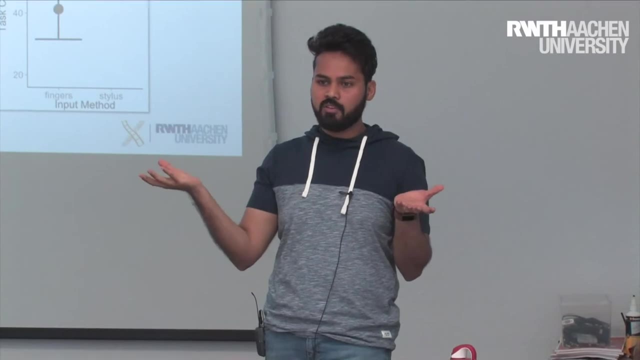 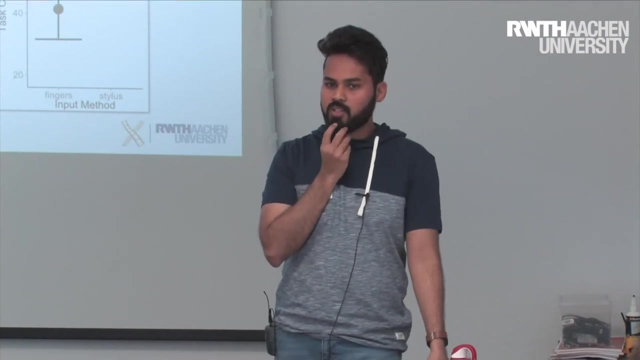 And visualization. I mean you can find which distribution is is better, right, You can find which distribution results in more typing speed based on the mean value and standard deviation. What can it not say? Is there a problem with this? So the problem with descriptive statistics and 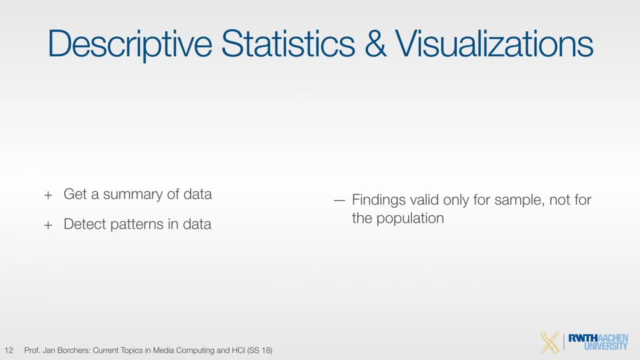 visualizations is that the findings that you make is only valid for the sample that you're collected. Right are billion people or two billion people in the world, right or how much, and you collect a sample of that. so if you collect like 30 people out of that, then 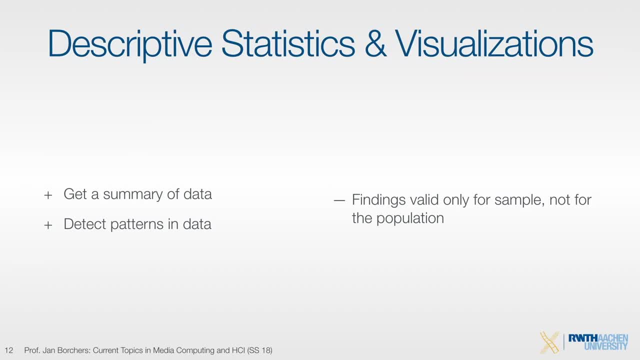 your findings are only valid for those 30 people, right? of course it is infeasible to to collect all the you know, to get all the users, to get all the entire population of the world to participate in your user study. that is infeasible. but there is a way to estimate that there is a way to from 40. 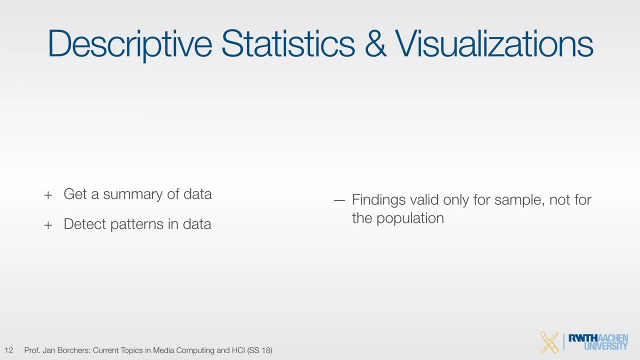 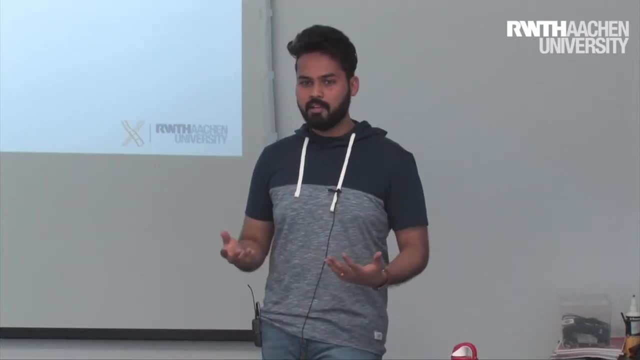 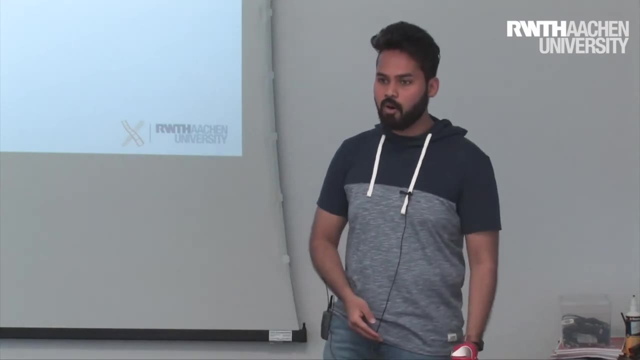 or 50 users. there is a way to estimate the population. okay, do you guys know this concept of population and sample from before? okay, so population basically means every subject there is. so in in our case, in our scenario, it will be all users in the world. if you are designing something for blind people, then there. 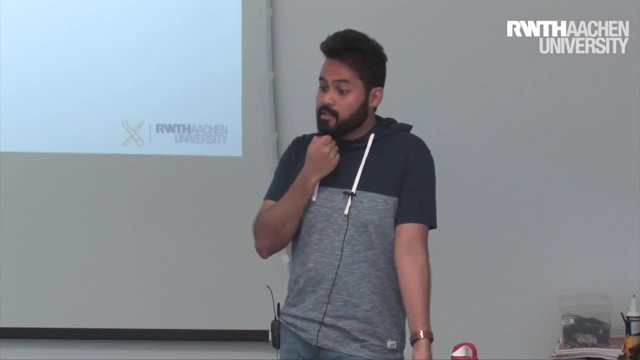 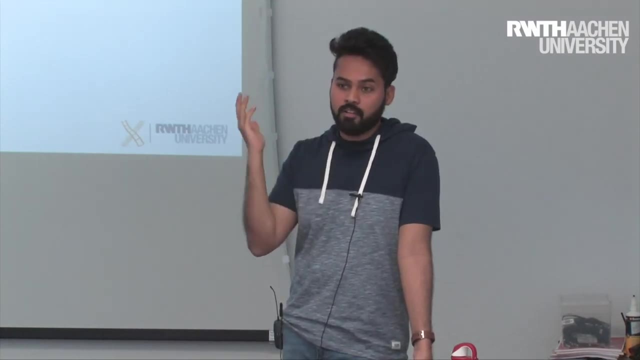 will be all the blind people in the world. you know people who are blind, people who are blind, people who are blind people. if you are testing something else, maybe you're designing, I don't know, an augmented reality headset for frogs. then the users, the population would be all.